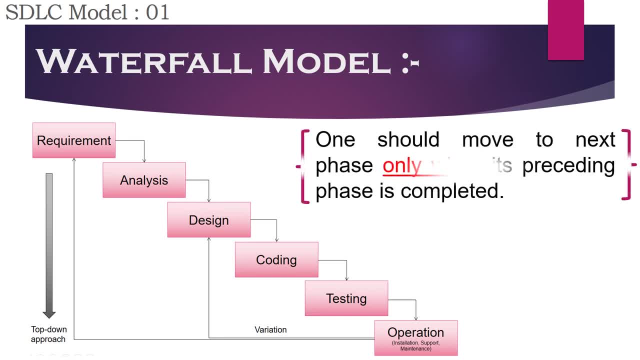 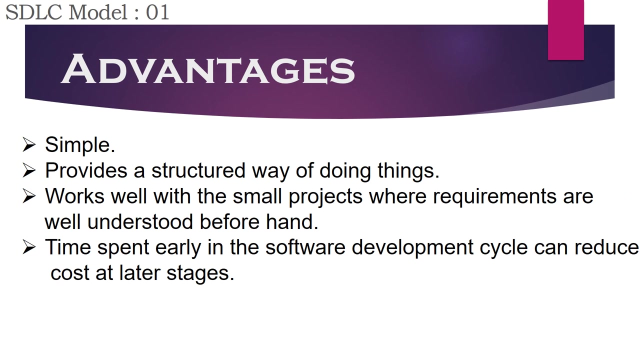 for software development. The central idea behind this model is one should move to the next level of software development, So means the next phase will start only when its preceding phase is completely reviewed and verified. There could be few advantages of this model Like it's very simple to understand as well as to execute. 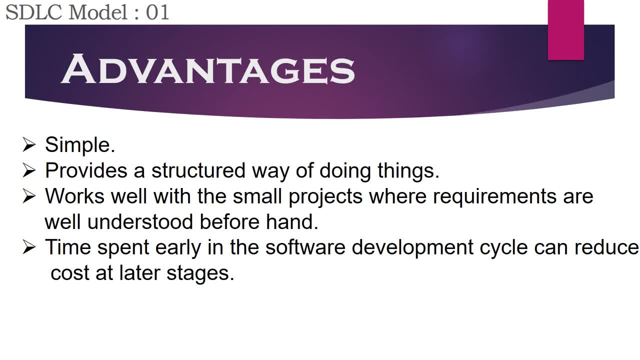 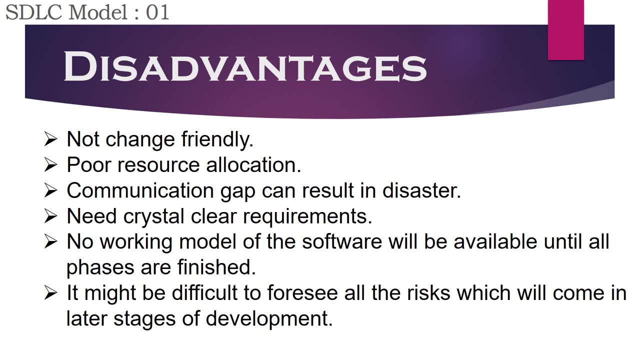 It works well with the small projects where a technology is well known, with no more surprises, And all the requirements are well understood beforehand. But largely while considering the complexity of today's software industry, waterfall model is not at all suitable and will have many disadvantages. 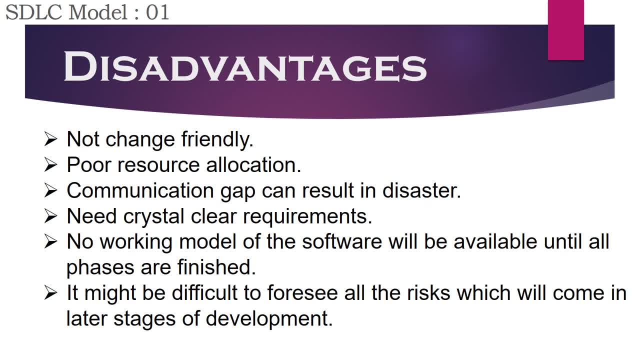 Like poor resource allocation- There will not be any working model of the software until all phases are done- And poor risk management. So let's try to understand a better version of waterfall model. So let's try to understand a better version of waterfall model. 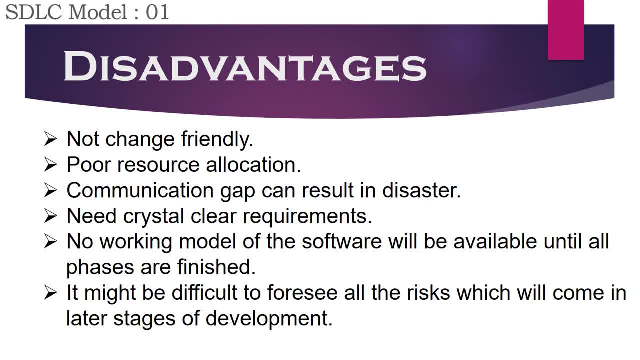 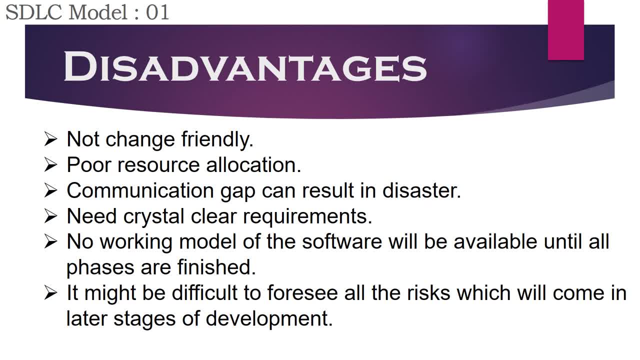 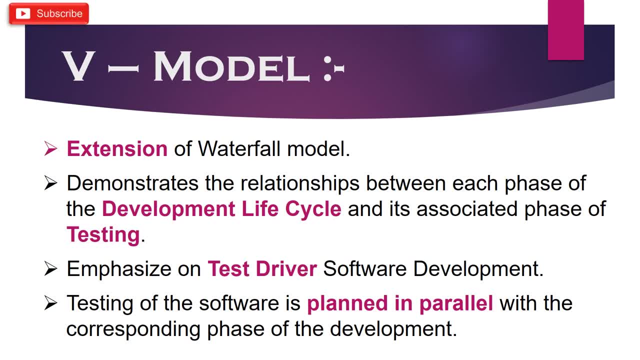 Which still has the rigidness of waterfall model, but emphasize more on software quality. So, friends, V model is an extension of Waterfall model which demonstrates the relationship between a phase of development life cycle and its associated phase of testing Means. in V model we will not only plan a development phase along with the development. 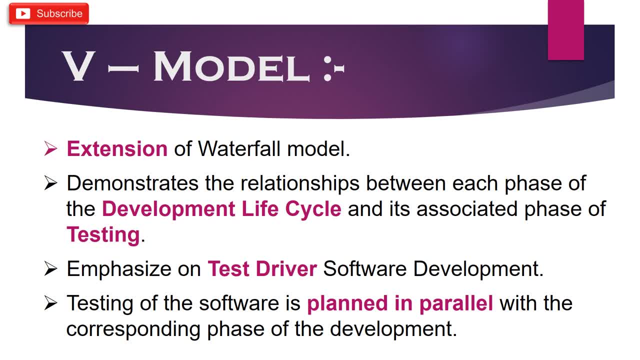 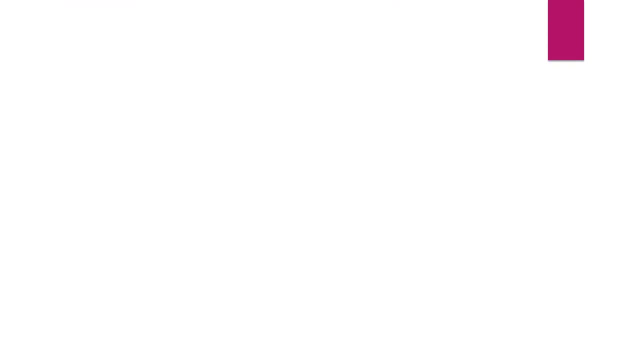 phase, its testing. So, in summary, testing of the software is planned in parallel with its corresponding development phase. Remember, I am using the word planned here. Testing will not be conducted, it will be just planned like writing: test cases, testing cost and time estimation. 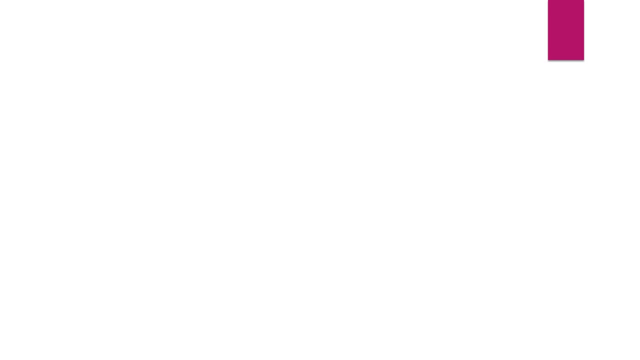 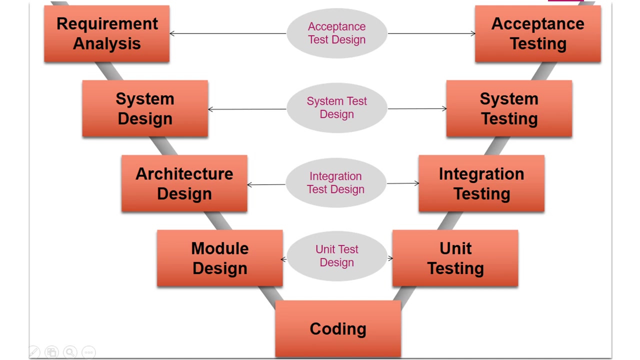 Let's look at the vModel in detail and discuss its various development phases. So here we go. Similar to waterfall, you can see. a linear approach in vModel also means the next phase will start only when its preceding phase is completed. All models start with the requirement phase. 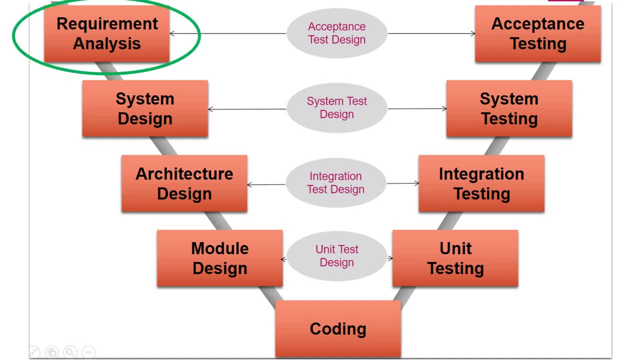 where the team or management tries to understand product requirements from customer perspective. So let's look at the vModel in detail and discuss its various development phases. This phase is concerned about establishing a mutual understanding that what the ideal system has to perform. However, it does not deal with the low-level details of how the 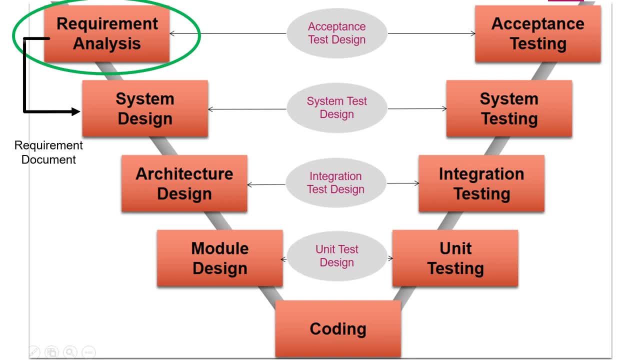 software will be designed. Mutually agreed requirement document will be the output of this phase. So once we got the clear and detailed product requirements, it's the time to analyze those requirements, conduct feasibility study and design the complete system. Output of this phase: the high-level system. 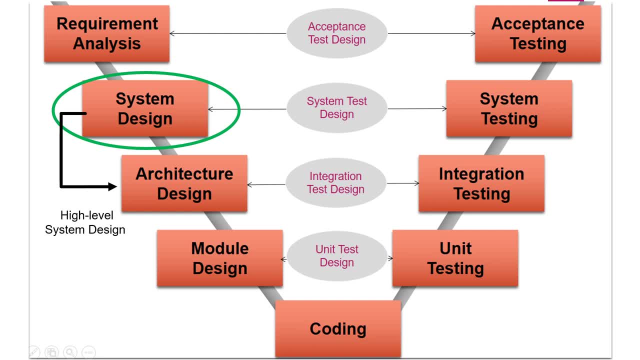 design document will have the complete picture of various components of the system, like user software, hardware interfaces and database. Now come the role of Software Architect Patient, who will analyze the system design document and generate high-level software design. He will take all the important steps in vModel. 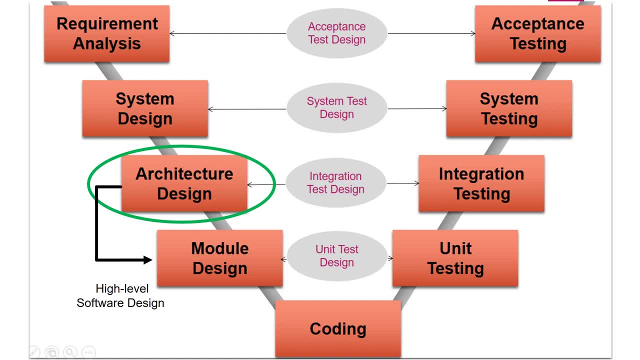 technical decisions in this phase, like which controller will be suitable, which programming language should be used, memory communication protocols and many more. Once the software blueprint is ready, software developer can start designing the individual modules and generate low level design documents. Then comes coding, where the actual construction of the software takes place. 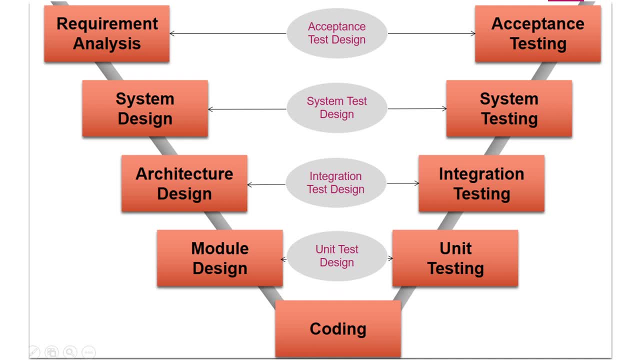 So, as we discussed earlier that in vModel the testing phase is also planned in parallel with its corresponding development phase. So before closing requirement phase, acceptance test should also be planned. Once the software is ready it will be tested by customer or system user for acceptance. 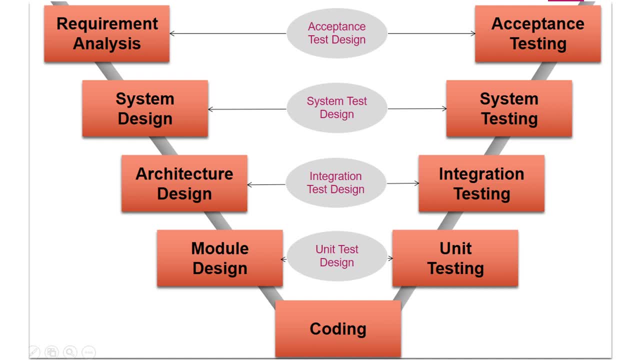 Similarly, system test specification and integration test specification will also be planned in parallel with the system and architecture design phase. System testing will be conducted just before the product delivery to test the entire system functionality, including all internal and external components. An integration test will be conducted to test the software, internal modules and internal